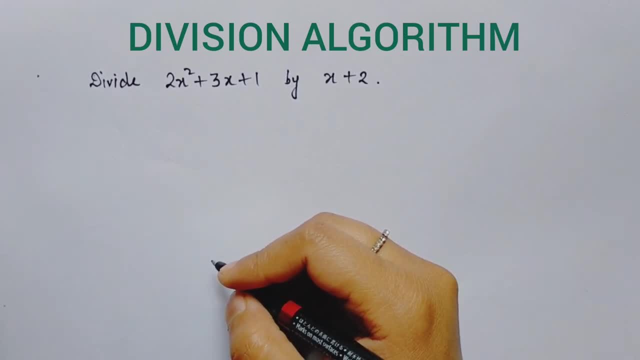 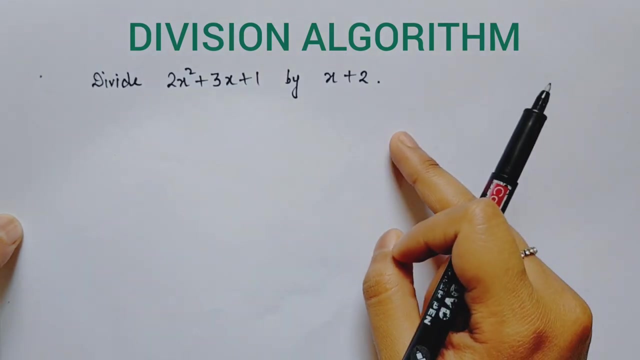 Since many students have problem in normal division of two polynomials, so here we will discuss how to divide one polynomial by another polynomial. So there is a simple method to divide and if you will learn how to divide then it will be very easy for you to solve. 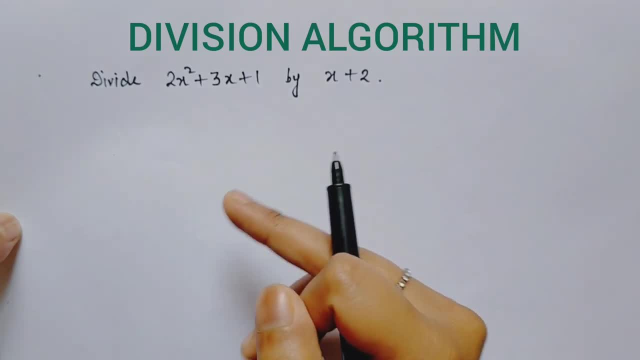 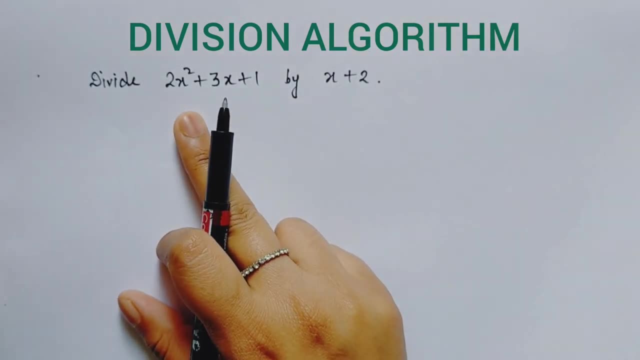 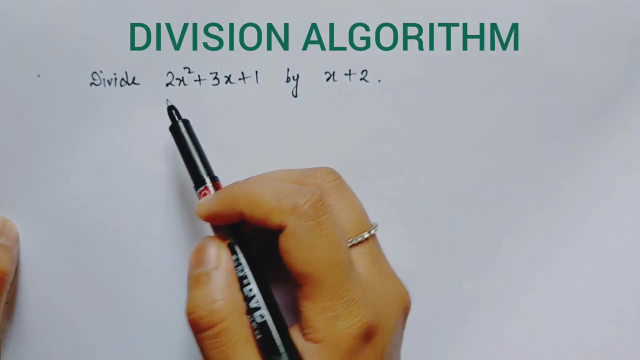 all questions of chapter polynomial of class 9th and also of class 10th. So this video is for all. So we will start now. how to divide. So first, what is the rule to see whether division is possible or not. So here, in order to divide first, we see degree of dividend, Dividend. 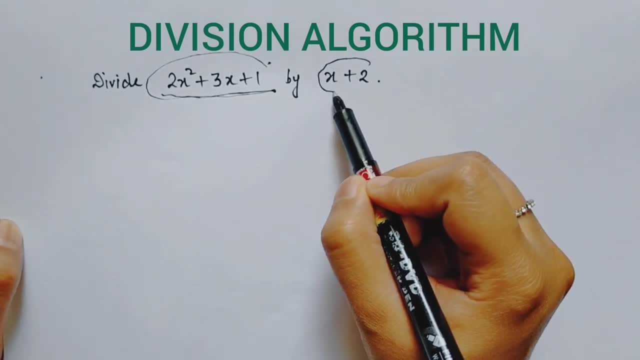 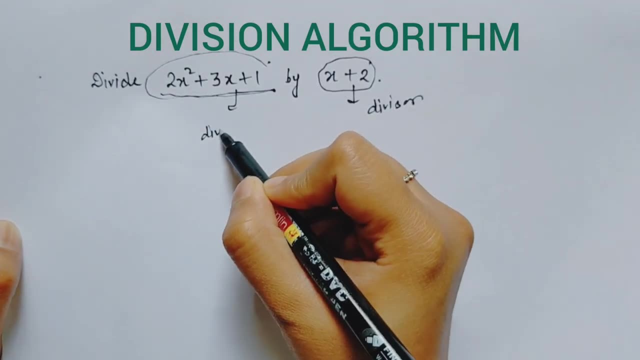 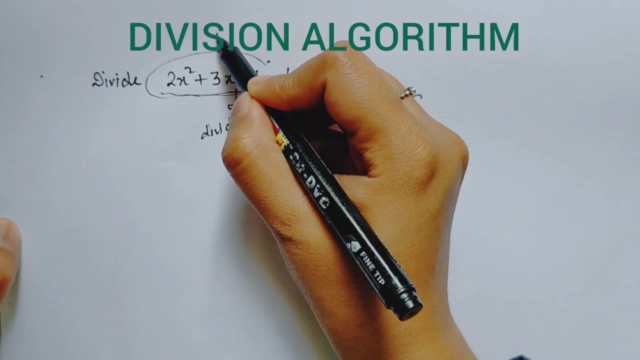 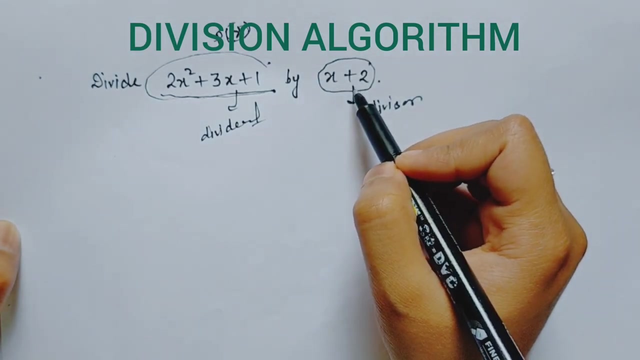 means we have to divide by another polynomial, x plus 2. It is divisor and this is dividend Dividend We generally We generally call dividend by px, means it is a polynomial of x variable, px, and it is also a polynomial of x variable. So we generally call divisor by gx. So it is a simple notation. 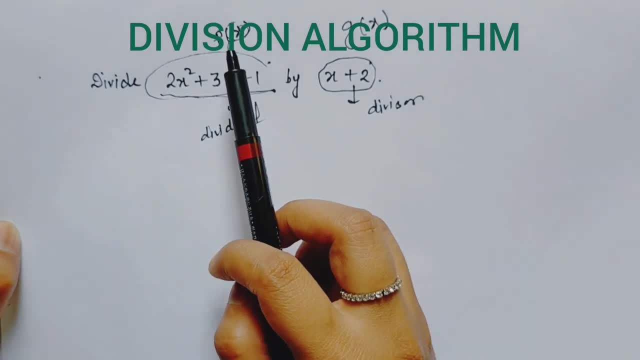 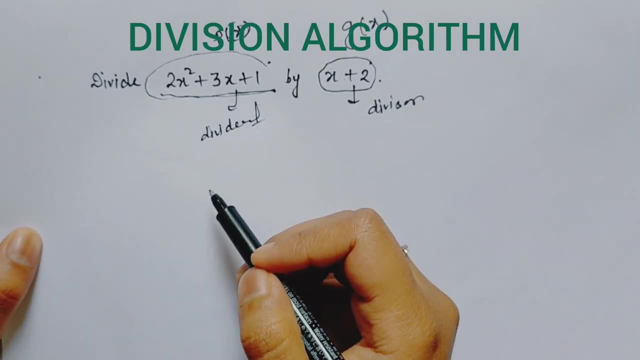 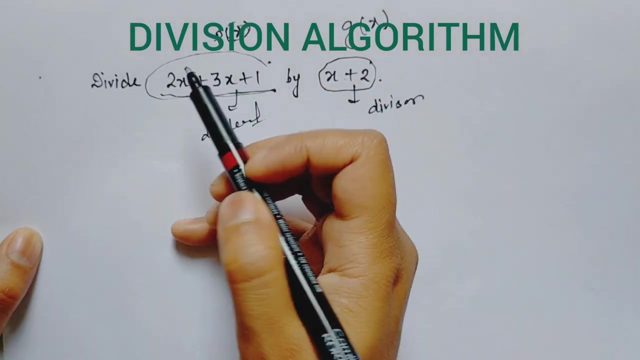 to represent dividend and divisor. So we will always represent dividend by px and divisor by gx. So in this video we will discuss how to divide normally. So first rule: I told you that first we see degree of dividend, It should be greater than degree of divisor. So here: 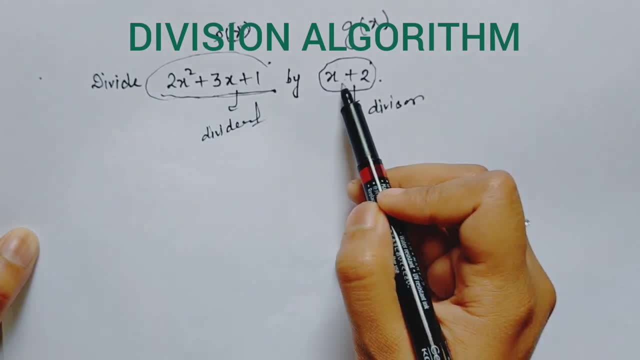 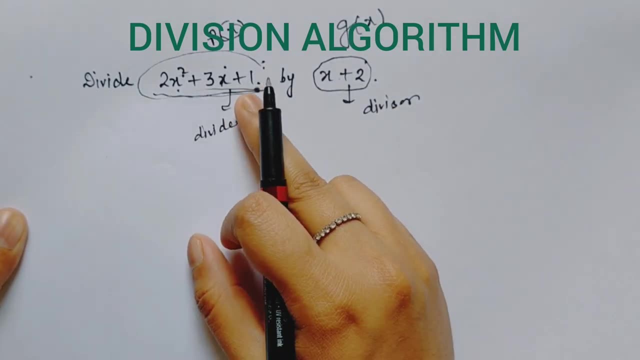 degree of this polynomial is 2, because highest power is 2.. And here degree of this polynomial is 1.. So since 2 is greater than 1, so we can divide this polynomial by this easily. Now, second: I skip this rule. First we will arrange them in standard form, So everything is already. done for you. So we will start division here. So how we start: Normally we keep dividend inside the scoring收ic. We should fällt the device within second column. So division is the last one. But if you will see here, first rule: First of all we have to divide every. 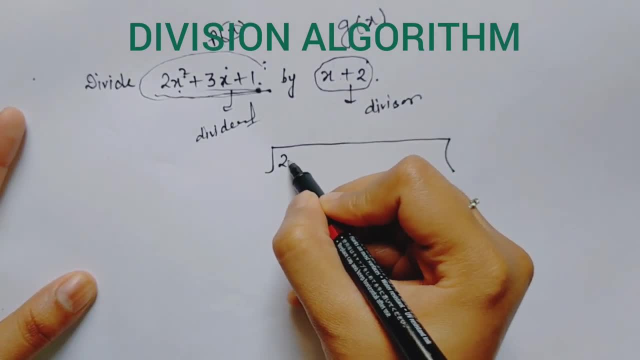 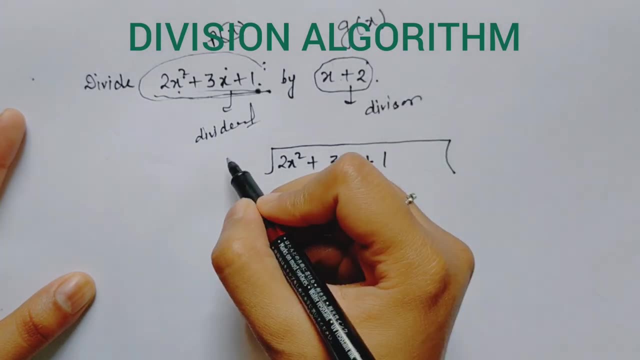 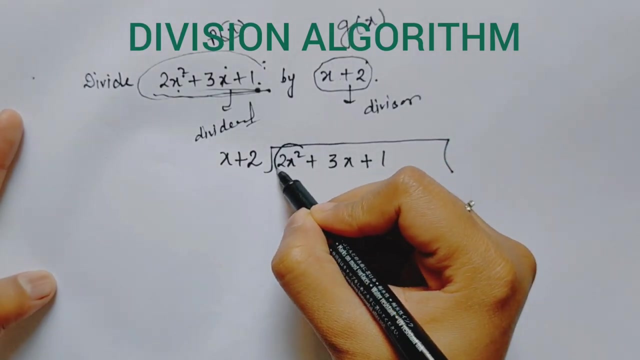 dividend by px. divi screaming is well known. Logically, this homonym of divi is. divide by px is the언 memorialize for subdivision. Dividend inside this bracket, divisor is always kept outside x plus 2.. Now what we do? first of all, we see first term of dividend and here first term of divisor. 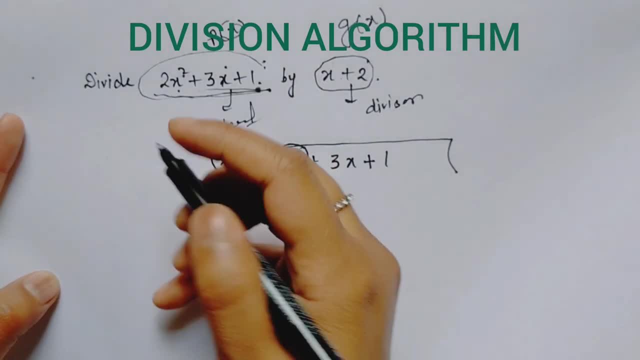 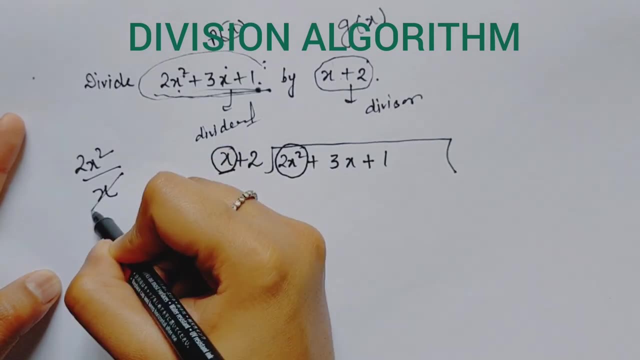 In rough. we will divide this term by this term, always, Always, always what we have to do: first term of dividend, we have to divide by first term of divisor. So when I will divide, x will be cancelled with this, I will get simple 2x. 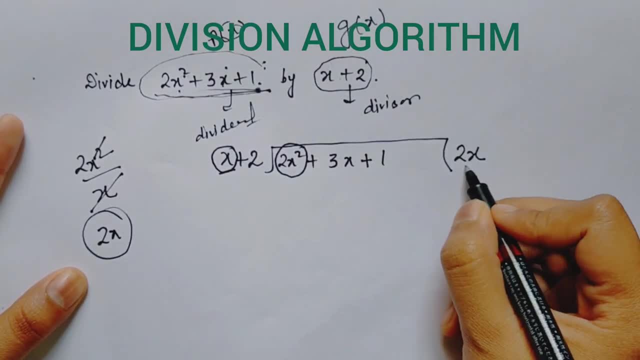 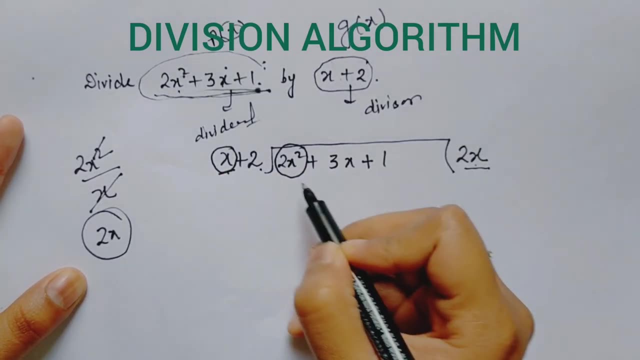 So I will write here: 2x. So first term will be obtained by dividing first term of dividend by first term of divisor. Now multiply 2x by both to write below. So 2x multiply x will give you 2x square. 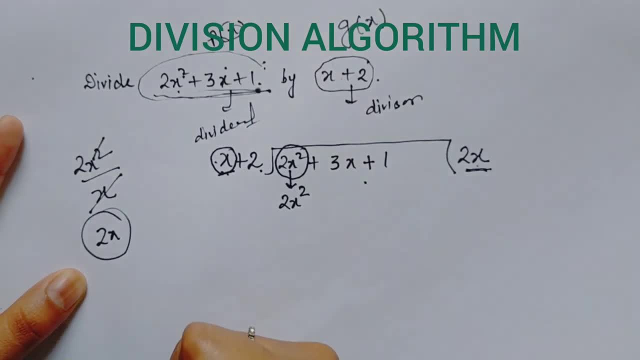 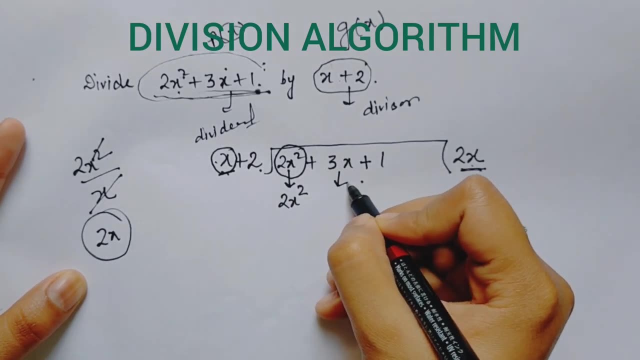 So 2x square exactly below x square term. So 2x into 2 will give you 4x, or here plus sign. so plus 4x exactly below 3x. So I got plus 4x. Now we always put a line. 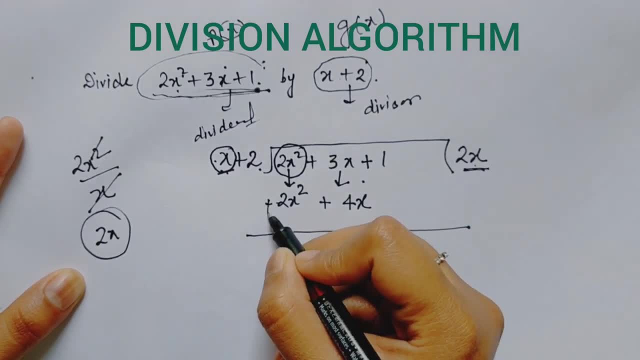 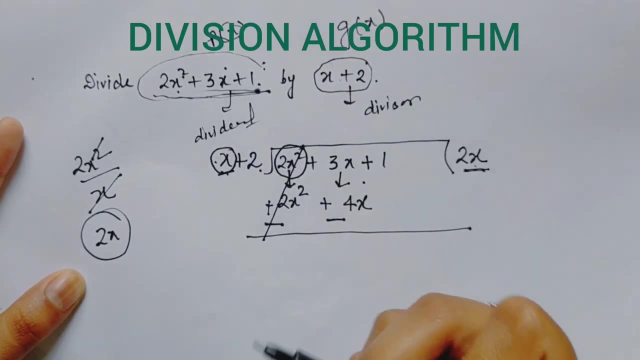 After line. we always change their sign. Here it was plus originally, so here will be minus sign. Plus will be converted into minus sign. Can I say these two terms will be cancelled. 2x square minus 2x square: it will give you 0.. 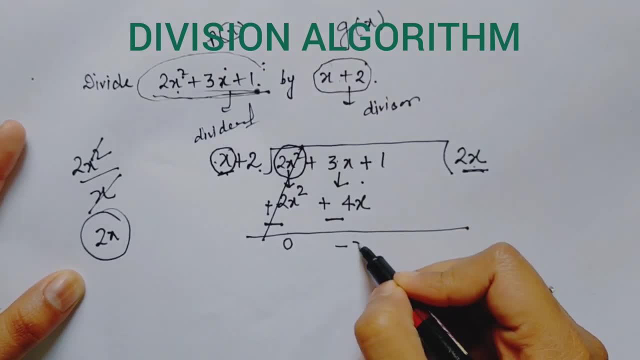 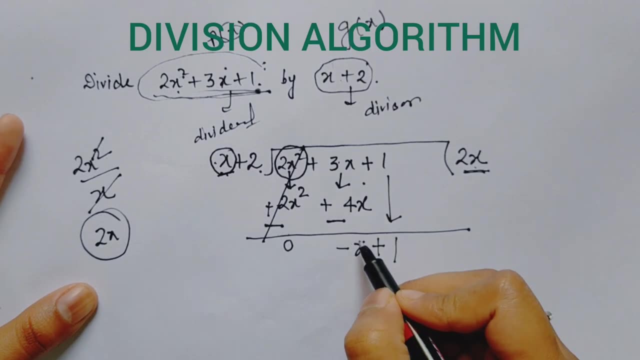 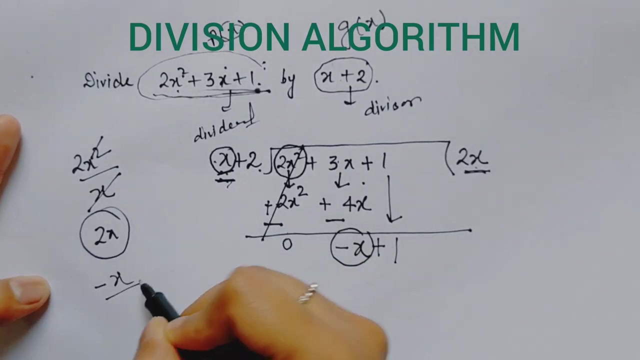 Now 3 minus 4, it will give me minus x. 1 will be noted as it is plus 1.. Now again, first term to be divided by same term of divisor. So in rough, minus x upon positive x. 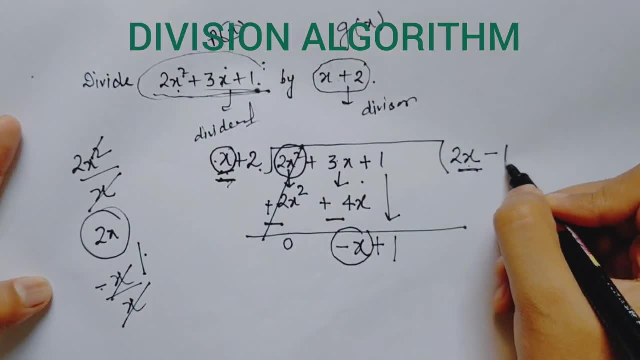 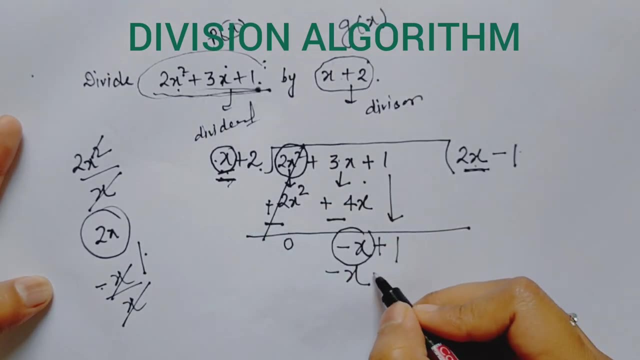 So it is 1, so minus 1 is next term of quotient. So minus 1 into x, minus x, Minus 1 into plus 2.. Minus 2.. So again I will put a line and change their sign. 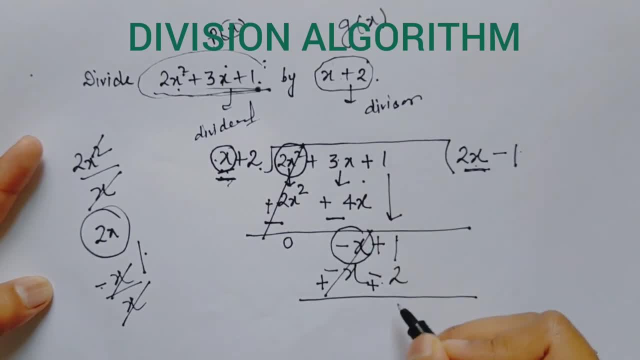 Plus plus, It will be cancelled, and 2 plus 1 will give me 3.. Now see here what is the degree of this polynomial Here: x to the power 0 is there. That means 1 tha jese ham. x to the power 0: likh sakte hai. 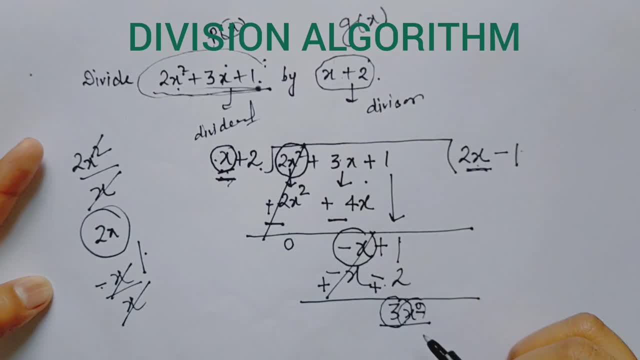 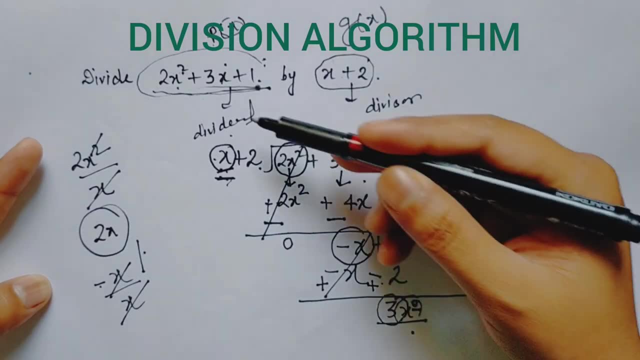 To jahaan par bhi x ki power less than divisor ho jaye wahi amara question stop ho jata hai. So here remainder has degree 0, while divisor has degree 1.. And 0 is there, So this is less than 1, so this is our remainder. 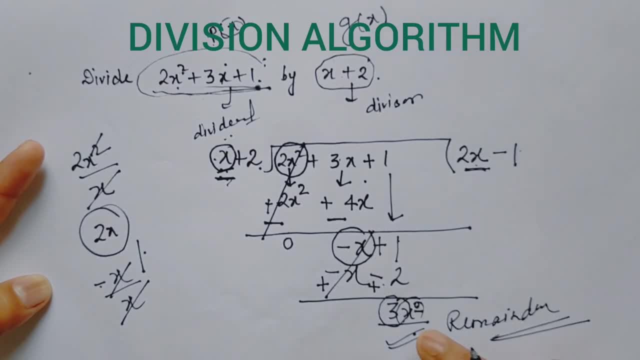 That means we cannot move further To yahaan par aapko yaad rakhna hai remainder ki degree agar apki divisor se kum aa jaye to aapka question, wahi stop ho jata hai. So here in this case 3x to the power, 0 means 3.. 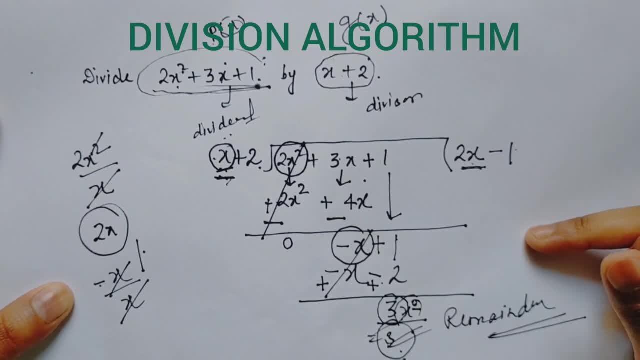 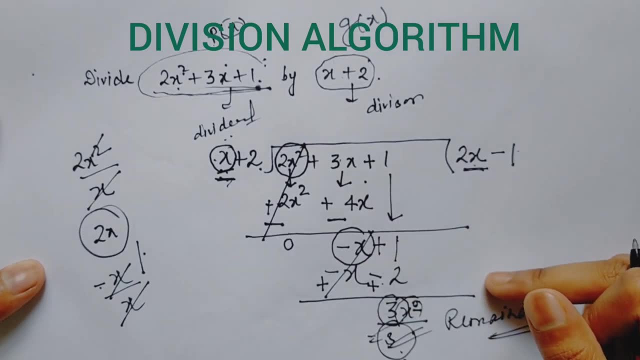 3 was my remainder. So this way we will divide all polynomials to get their quotient or their remainder. Jo bhi aap se poochha jaye, you can easily find out. Now, on the basis of this, you can try easily questions given on. 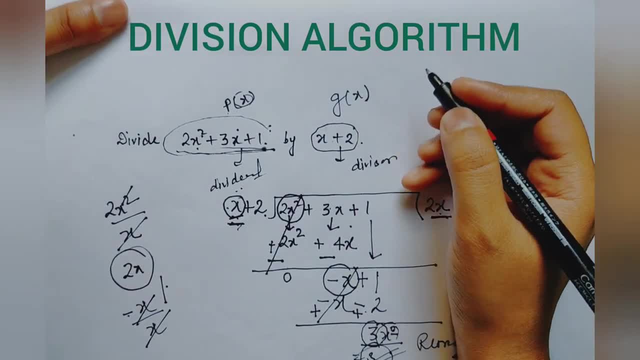 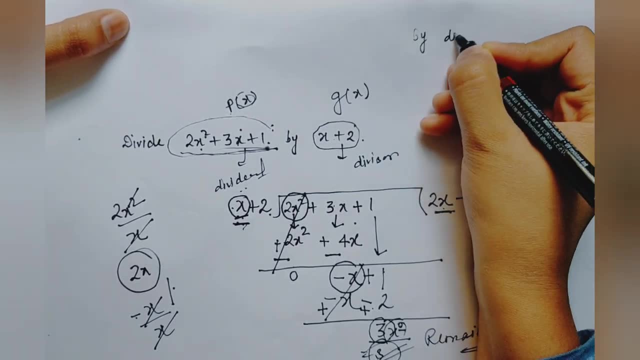 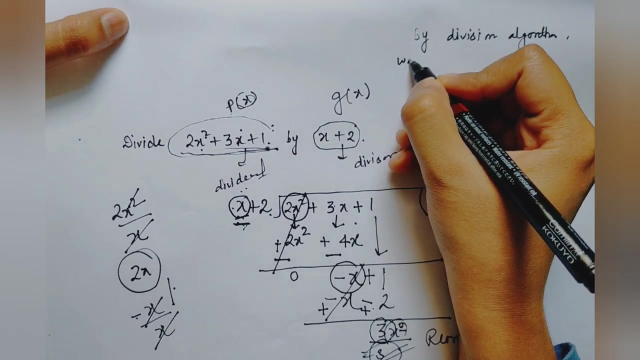 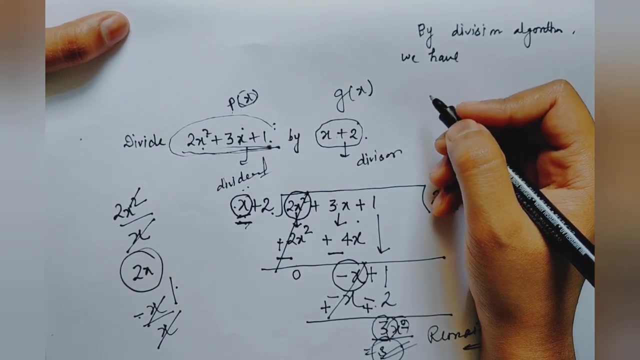 division rule. Now we will verify division algorithm. Since our solution is complete, the only need is to verify So by division algorithm we have. So what was the statement of division algorithm? It was: dividend is equal to divisor into quotient plus remainder. 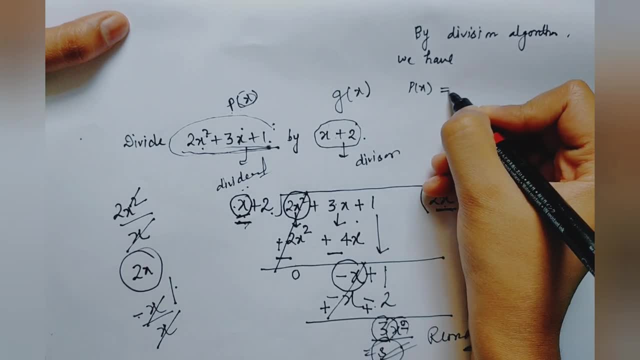 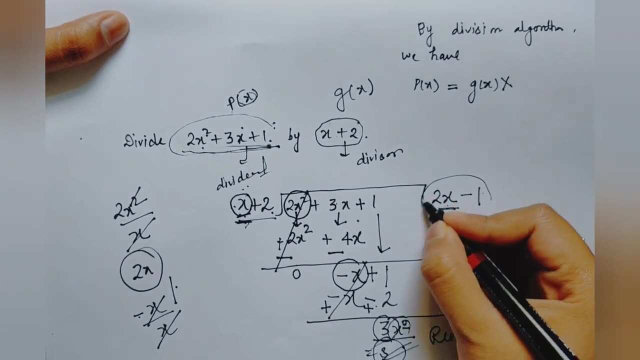 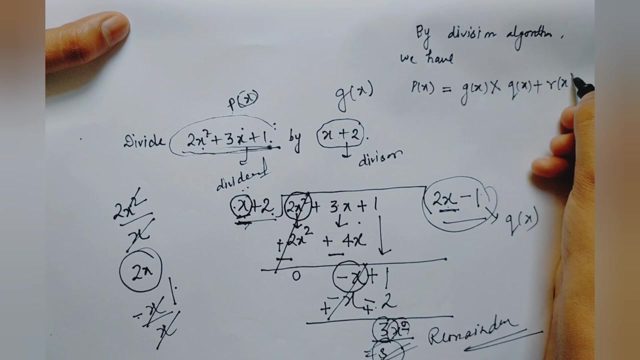 And dividend. always, px is equal to divisor. So this is the statement of division algorithm. Divisor is gx. gx into quotient Quotient is always represented by qx plus remainder rx. So we will verify this relation to complete our question. So px is already given this. 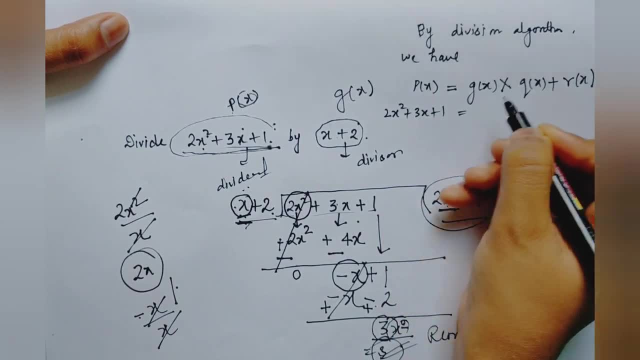 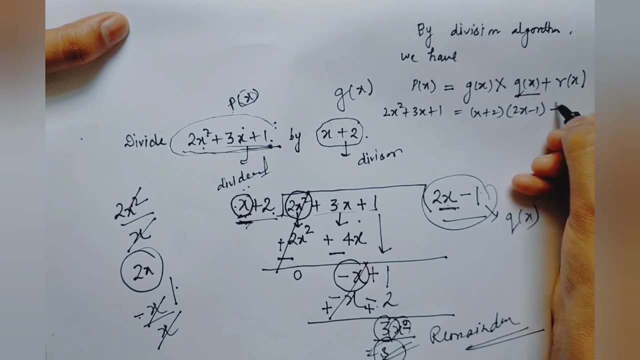 So 2x square plus 3x plus 1 is equal to gx means x plus 2. in multiplication with qx means 2x minus 1.. Plus rx, rx means remainder. that was 3.. So I will prove: left is equal to right. 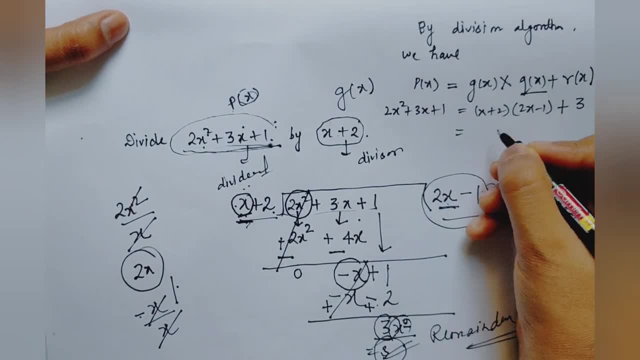 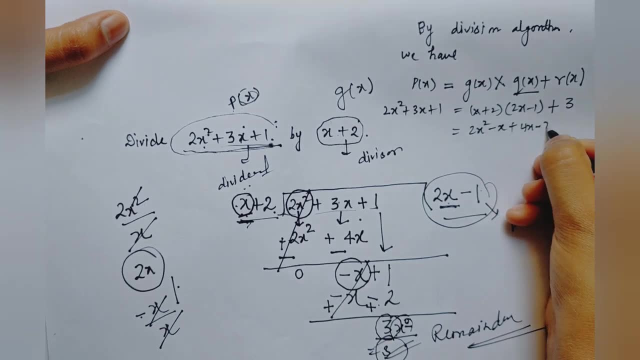 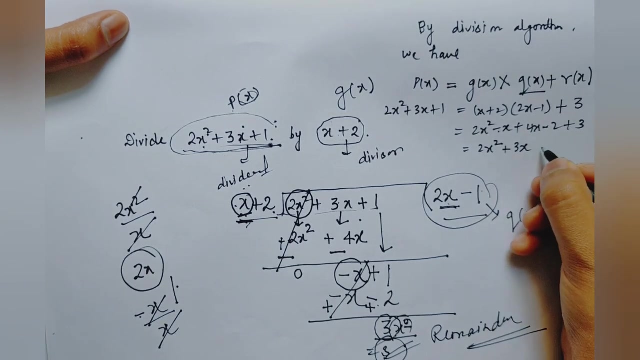 This left side is equal to right side. to complete my answer, So let's multiply 2x square minus x plus 4x minus 2 plus 3.. That is equal to 2x square 4x minus x plus 3x and 3 minus 2 plus 1.. 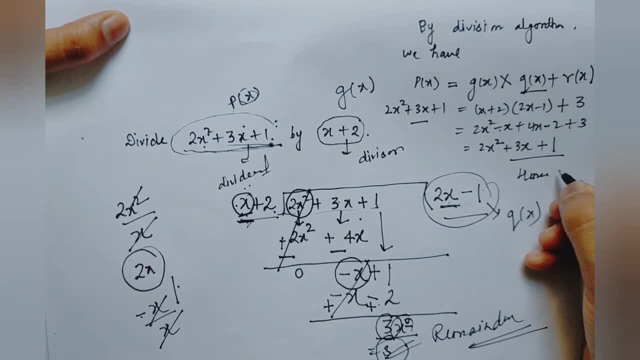 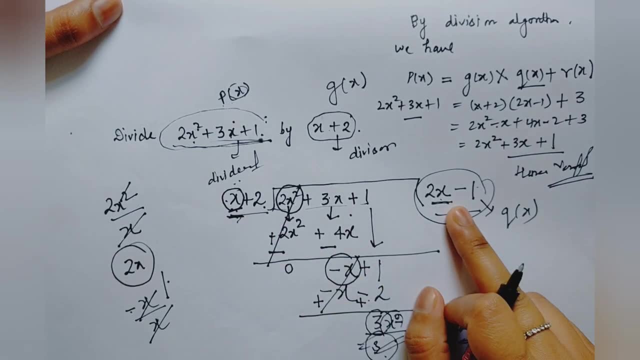 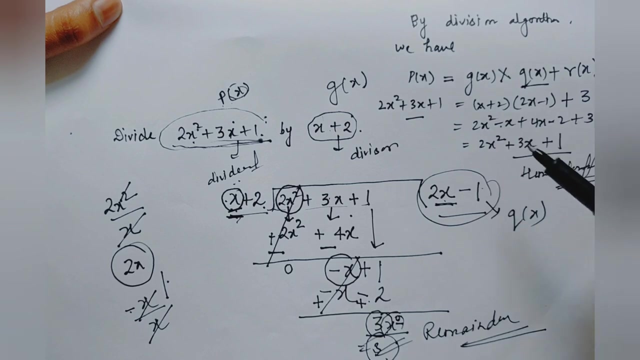 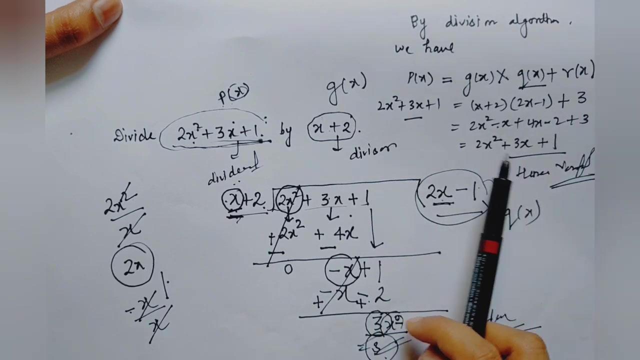 See, left side is equal to right side, Right side here, hence verified. So this way: first we will find out our quotient by dividing and we will also find out remainder. After that we will use division algorithm to prove our relation. So, after writing everything in place of px, gx, qx and rx, we will solve it further to get right side equal to left side. 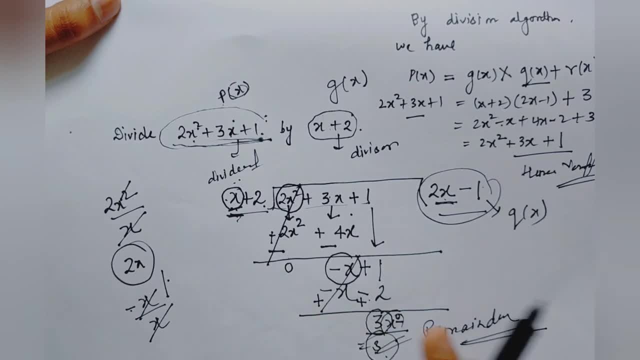 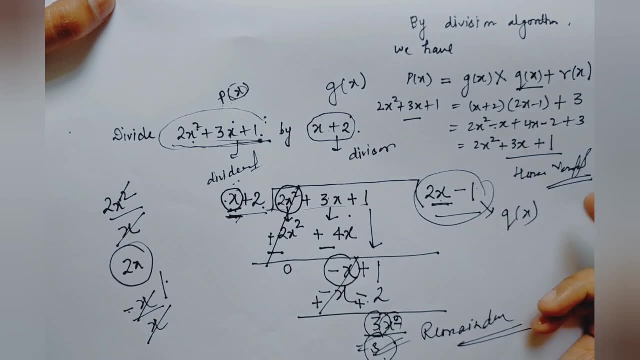 So this is the complete solution of division algorithm given in your NCIT book as example and also as exercise question. So whenever you have problem in solving other questions also, you can comment in the given comment section. So thank you, Thank you. 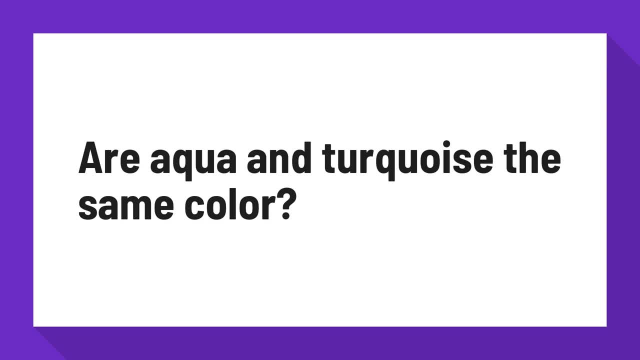 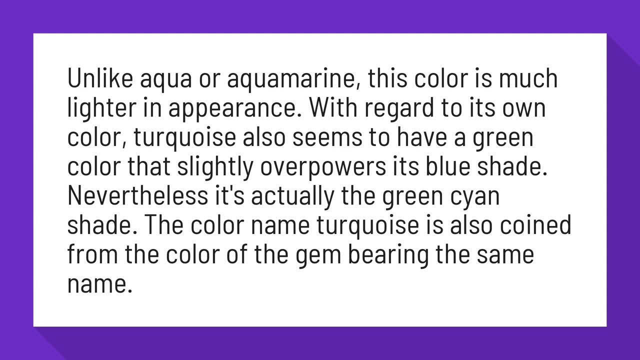 are aqua and turquoise the same color? unlike aqua or aquamarine, this color is much lighter in appearance. with regard to its own color, turquoise also seems to have a green color that slightly overpowers its blue shade. nevertheless, it's actually the green, cyan shade. 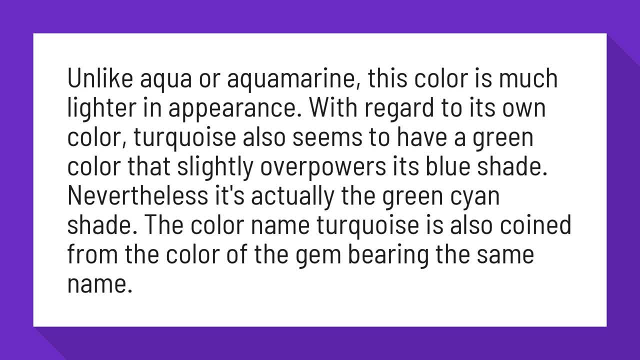 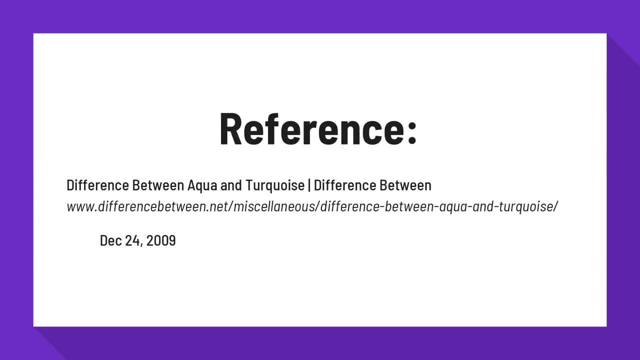 the color name turquoise is also coined from the color of the gem bearing the same name. thanks for watching. please subscribe. 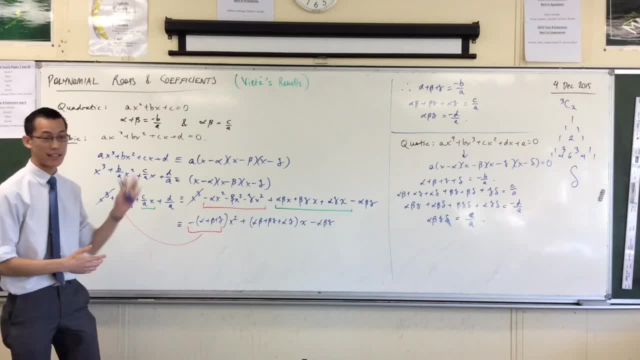 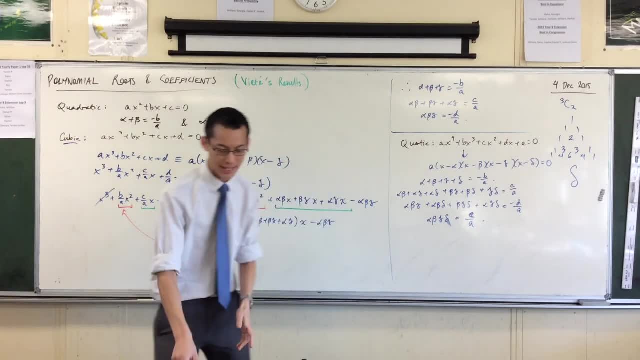 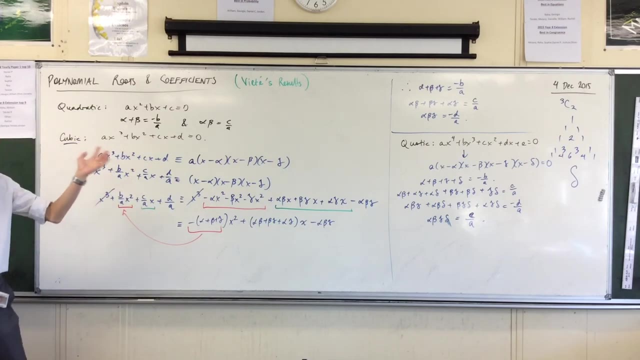 Now, from all of this, what this tends to transition to is a bunch of questions in manipulating and combining these different results in different ways. I will show you those examples in a second, but I have to justify for you, and I've got two big reasons why any of this is. 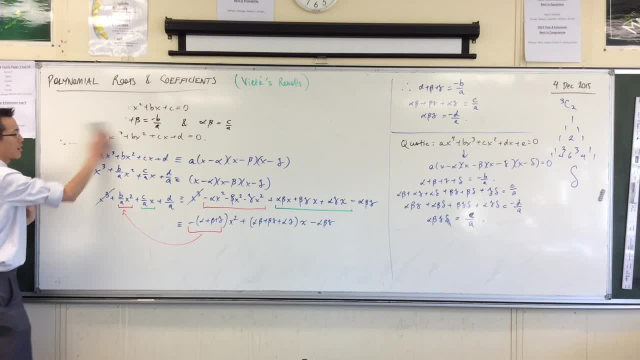 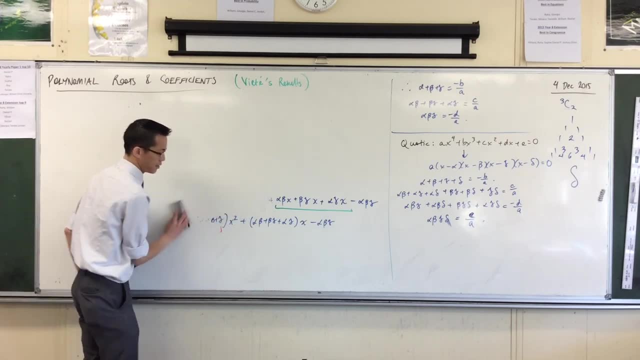 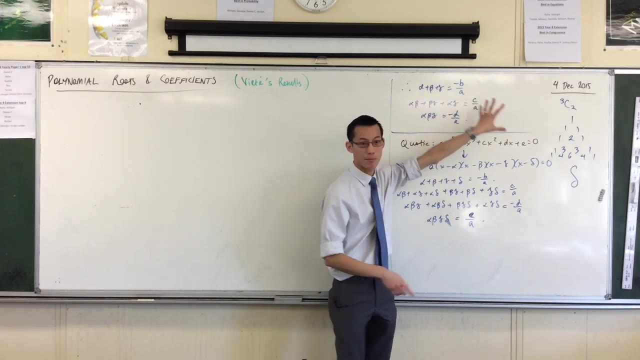 What's the point of all this? Why do we bother learning this? I've got three reasons for you. The first reason: I just need a bit of space here. The first reason is what we're saying here is we know these relationships between what these roots are, and we can get them very, very simply. 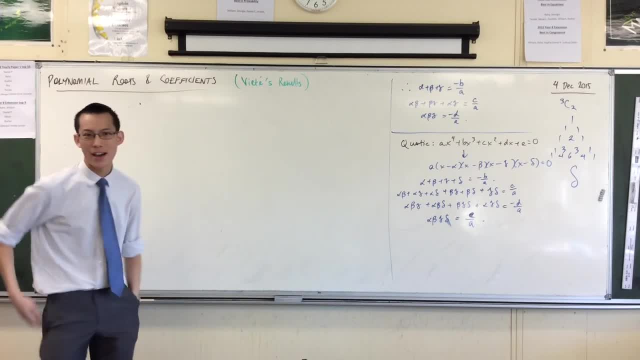 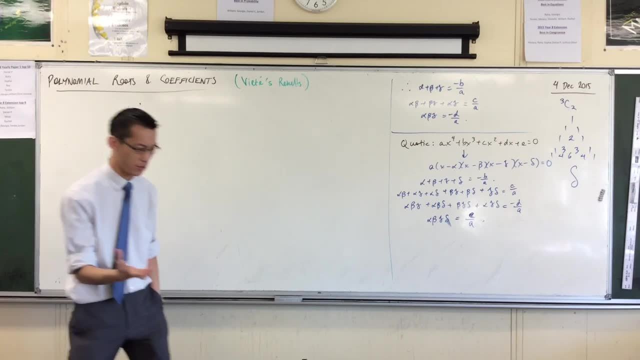 Like you just have to read off what the coefficients are and divide a pair of numbers Like how easy does it get? Now the enormity of that is probably lost on you a little bit, because we're quite used to finding roots and knowing what they are.